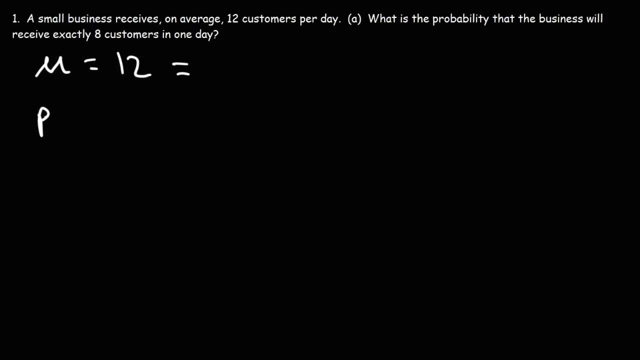 symbol here Now to calculate the probability. we're going to use this formula. Capital X is the random variable. Lowercase x, in this case is 8.. That's the probability that we're trying to calculate. We want to know what's the. 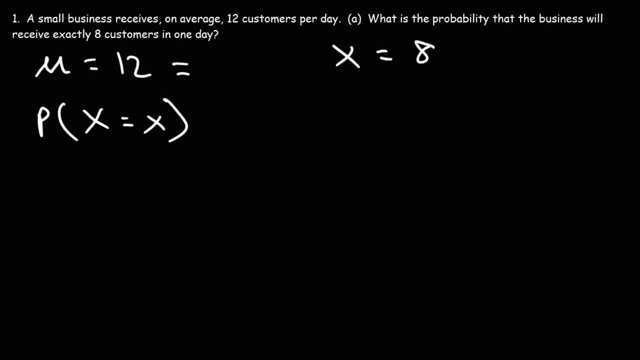 probability that the business will receive exactly 8 customers in one day. So x is 8.. And the formula is: mu raised to the x, e to the negative, mu divided by x- factorial. So let's replace lowercase x with 8.. So this is going to be 12 raised to the 8, e to the 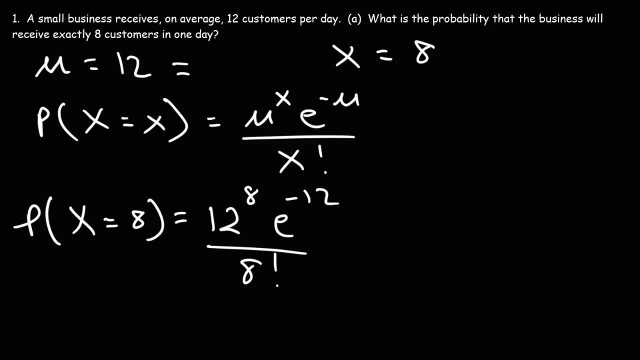 to the negative 12 divided by a factorial. Now, keep in mind: e is the inverse of the natural log function and e is basically a number. It's 2.71828.. 8 factorial, that's 8 times 7 times 6. 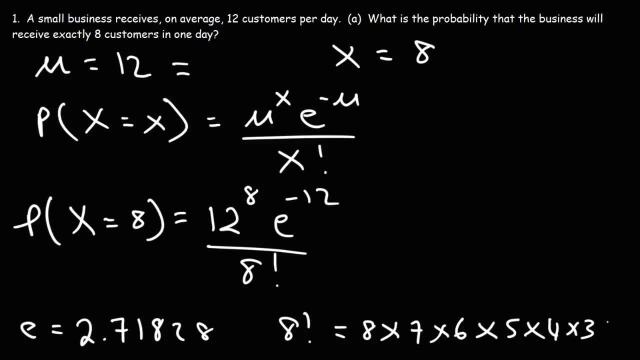 times 5, all the way to 1.. So if you were to plug this into your calculator, you should get hold on one second. You should get 0.065523, which, if we multiply that by 100%, that's approximately 6.55%. So that's the probability that 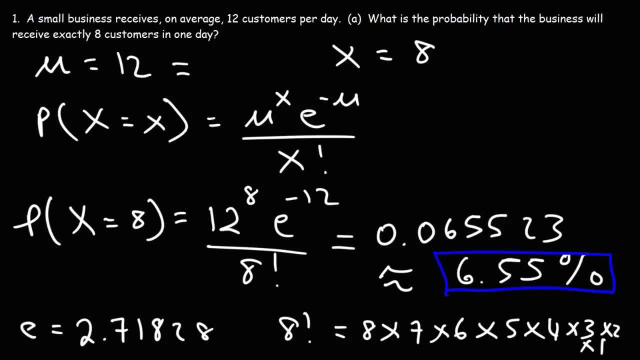 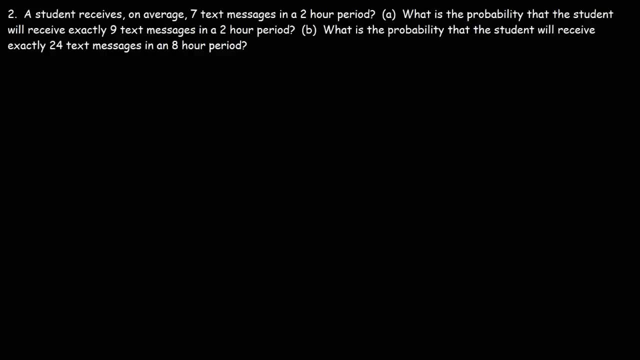 this business will receive exactly 8 customers in the next 10 years, So if you were to plug this into your calculator, you should get hold on 1 day. Number two: a student receives on average seven text messages in a two-hour period. 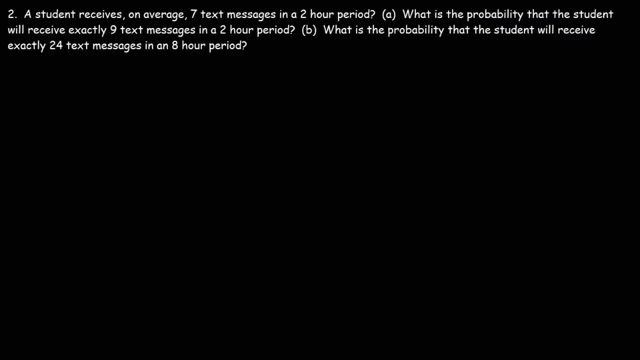 What is the probability that the student will receive exactly nine text messages in a two-hour period? So what do you think we have to do in order to solve this problem? Go ahead and try it Now. there's something that you need to pay attention to. 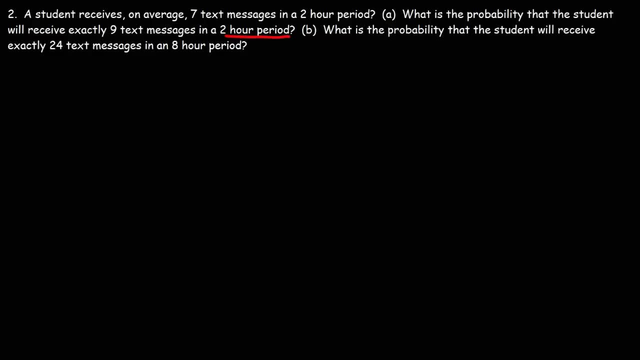 and it's the time interval. Notice that the time interval it doesn't change, It's the same. So therefore, seven is the mean. Now the only other thing that we need to find is x. We can clearly see that x is nine, because we want to calculate the probability that the student will receive. 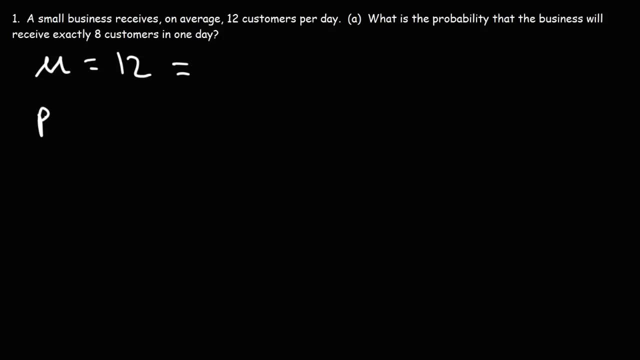 symbol here Now to calculate the probability. we're going to use this formula. Capital X is the random variable. Lowercase x in this case is 8.. That's the probability that we're trying to calculate. We want to know what's the probability. 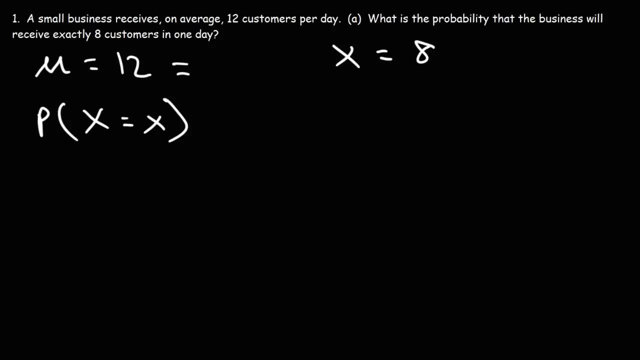 that the business will receive exactly 8 customers in one day. So X is 8.. And the formula is: mu raised to the X, e to the negative mu divided by X- factorial. So let's replace lowercase X with 8.. So this is going to be 12 raised to the 8,. 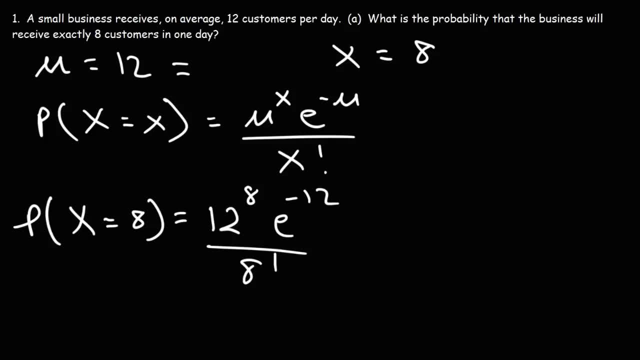 e to the negative 12, divided by 8 factorial. Now, keep in mind, e is the inverse of the natural log function And e is basically a number: It's 2.71828.. 8 factorial, that's 8 times 7 times 6 times 5, all the way to 1.. So if you were to plug this into your calculator, 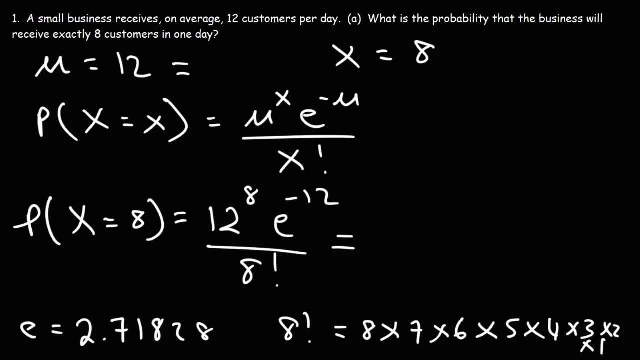 you should get 0.065523, which, if we multiply that by 100%, that's approximately 6.55%. So that's the probability that this business will receive exactly 8 customers in one day. So that's the probability we're talking about. That means that in the first problem it will give something. 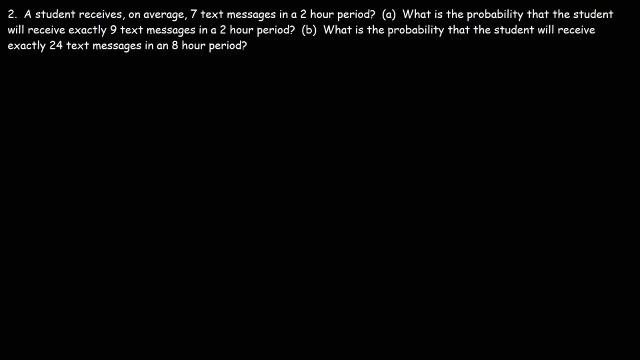 like this. Number two: a student receives on average, seven text messages in a two-hour period. What is the probability that the student will receive exactly nine text messages in a two hour period? So what do you think we have to do in order to solve this problem? Go ahead. 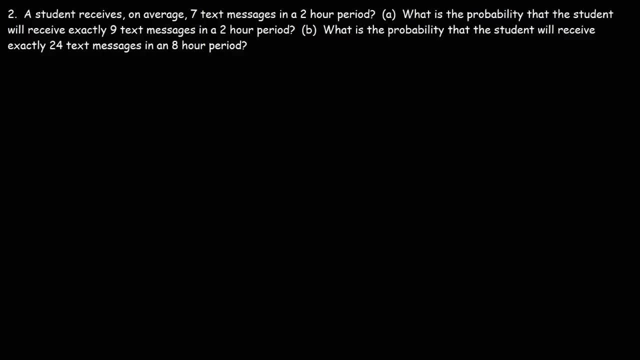 and try it Now. there's something that you need to pay attention to Now we want to to pay attention to, and it's the time interval. Notice that the time interval, it doesn't change, It's the same. So, therefore, 7 is the mean. Now the only other thing that we need to find is x. 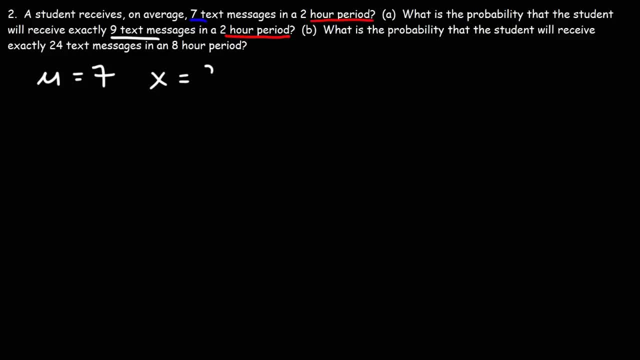 We can clearly see that x is 9 because we want to calculate the probability that the student will receive exactly 9 text messages in that two-hour period. So we need to calculate p when x is 9.. So let's go ahead and plug everything in. 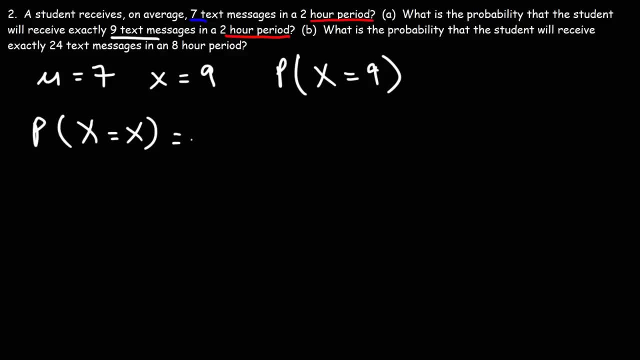 First let's write the formula. So, as we said before, it's mu raised to the x, e raised to the negative mu divided by x factorial. So x is 9, mu is 7.. So this is going to be 7.. 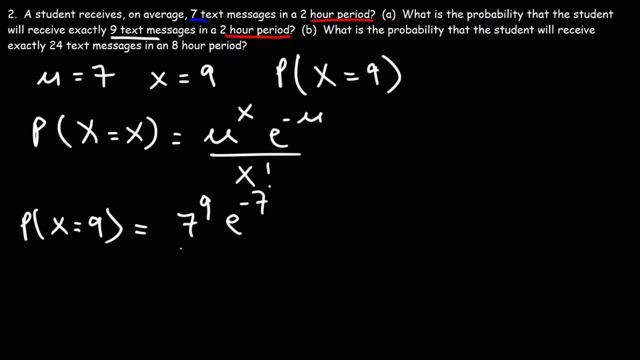 7 to the 9th power, e raised to the negative 7, divided by 9 factorial. So let's type that in, So you should get 0.1014,, which correlates to approximately 10.14%. So that's the answer for part A. 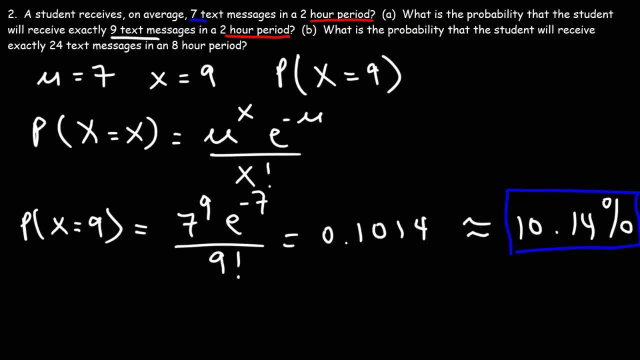 Okay, Now let's move on to part B, But first let's get rid of this information: What is the probability that the student will receive exactly 24 text messages in an eight-hour period? So notice, this time the time period is different. 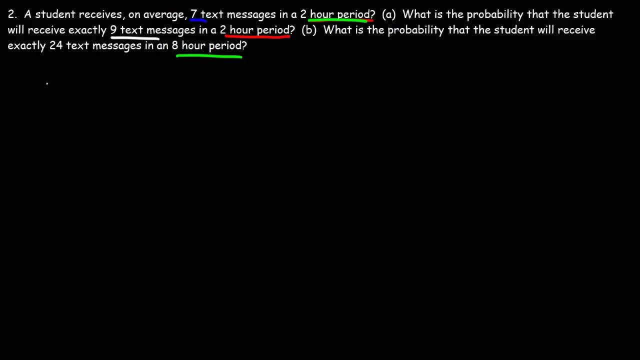 So therefore, the mean is going to change. The mean was 7.. What is the new mean value when the time period is 8 hours? So by looking at these values, you can see what it is. To go from 2 to 8, you need to multiply the 2 by 4.. 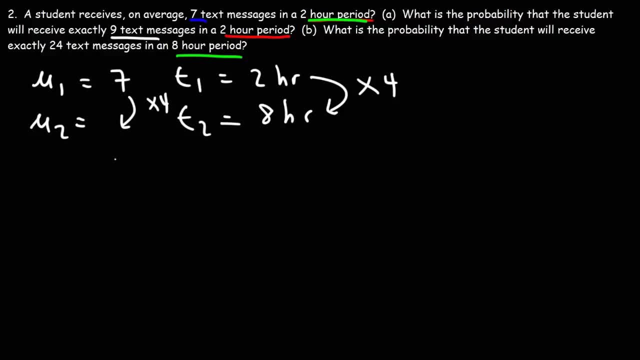 So, therefore, you need to multiply the mean by 4, which will give you 28.. 7 times 4 is 28.. So that's the new mean value. Now, sometimes the math will not work. It will not work out as nicely as what we see here. 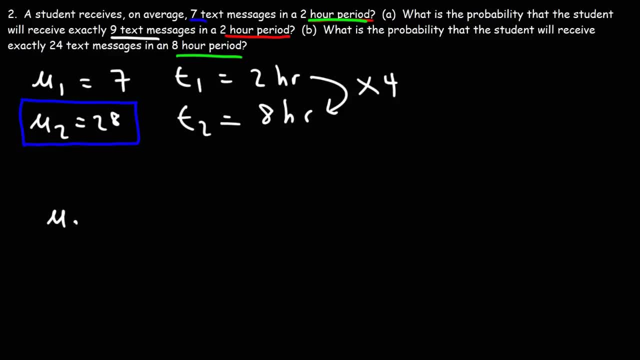 So you could set up a proportion. If you want a formula to do this, you can use this one: Mu 2 over Mu 1 is going to be T2 over T1.. So we're trying to calculate Mu 2, which is well. we're going to see that it's 28.. 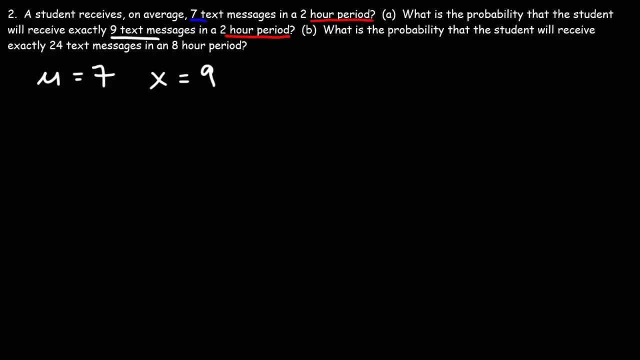 exactly nine text messages in that two-hour period. So we need to calculate p when x is nine. So let's go ahead and plug everything in. First let's write the formula. So, as we said before, it's mu raised to the x, e raised to the negative, mu divided by x factorial. 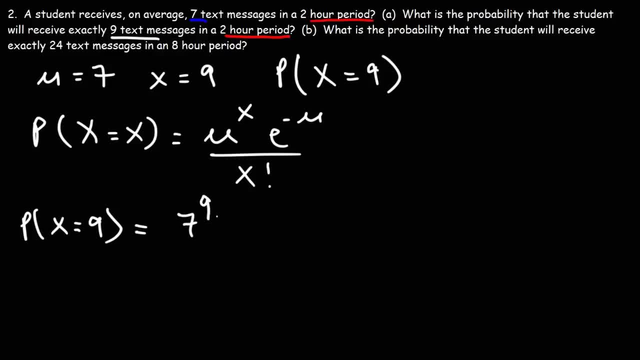 So x is nine, mu is seven, So this is going to be seven. to the ninth power, e raised to the negative seven divided by nine factorial. So let's type that in, So you should get 0.1014, which correlates to approximately 10.14%. 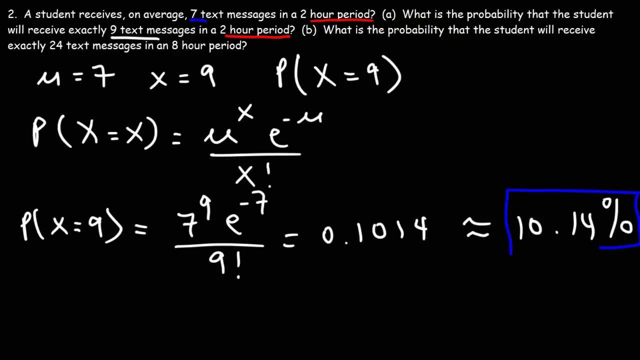 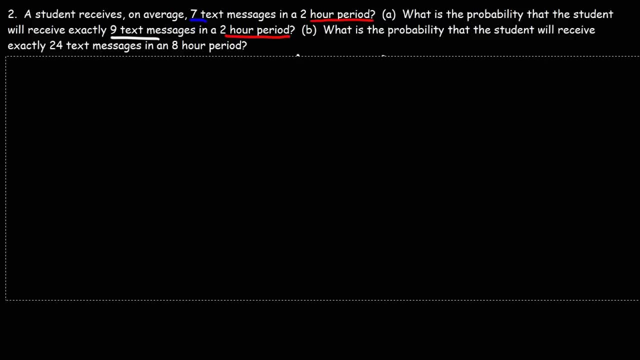 So that's the answer for part A. Now let's move on to part B, But first let's get rid of this information: What is the probability that the student will receive exactly 24 text messages in an eight-hour period? So notice, this time the time period is different. So therefore, 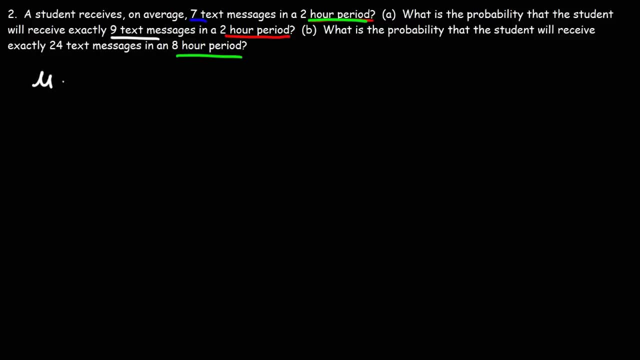 the mean is going to change. The mean was seven when a time period was two hours. What is the new mean value when a time period is eight hours? So by looking at these values, you can see what it is To go from two. 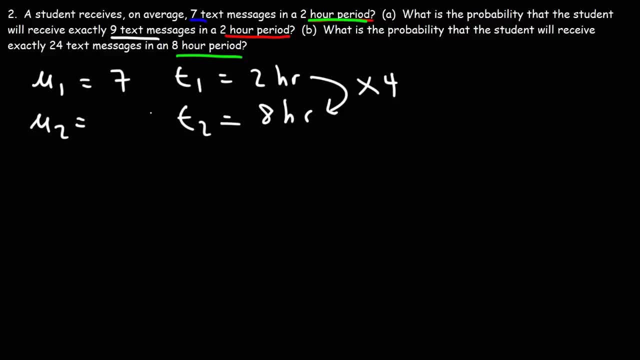 to eight. you need to multiply the two by four. So therefore you need to multiply the mean by four, which will give you 28.. Seven times four is 28.. So that's the new mean value. Now, sometimes the math will not work out as nicely as what we see here, So you could set up: 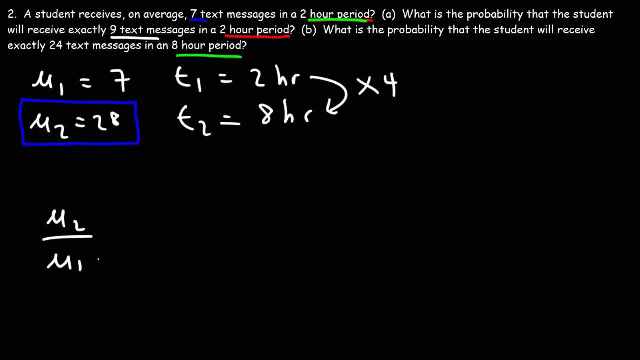 a proportion. If you want a formula to do this, you can use this one. Mu two over mu one is going to be T two over T one, So we're trying to calculate mu two, which is well, we're going to. 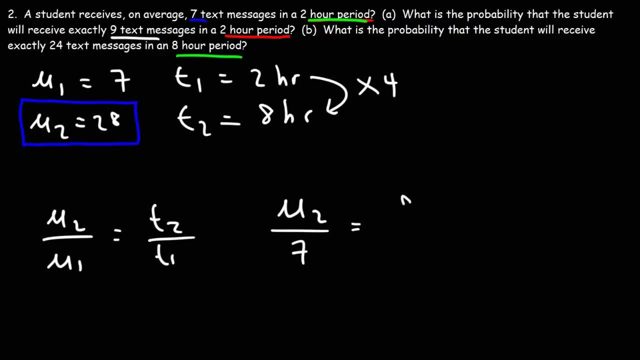 see, that's 28.. Mu one is seven, T two is eight, T one is two. So let's cross, multiply Seven times six is 56. And this is going to be two times mu two. Dividing both sides by two, we get 56 divided. 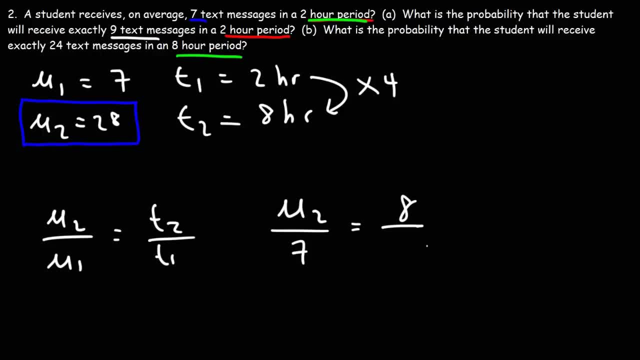 Mu 1 is 7.. T2 is 8.. T1 is 2.. So let's cross. multiply 7 times 8 is 56. And this is going to be 2 times Mu 2.. Dividing both sides by 2, we get 56, divided by 2, which is 28.. 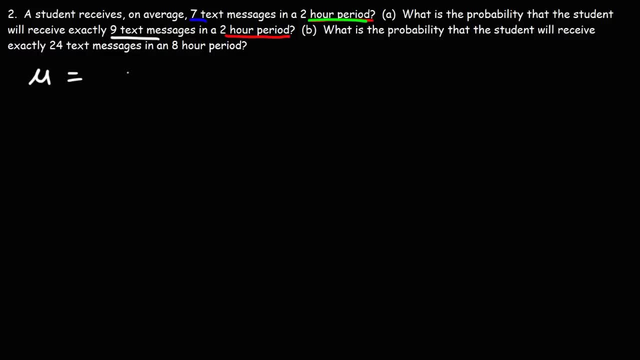 Now let's rewrite what we know. So, Mu, we could see that it's 28. And X has to be 24.. We want to calculate the probability that the student will receive exactly 24 text messages in this 8-hour period. 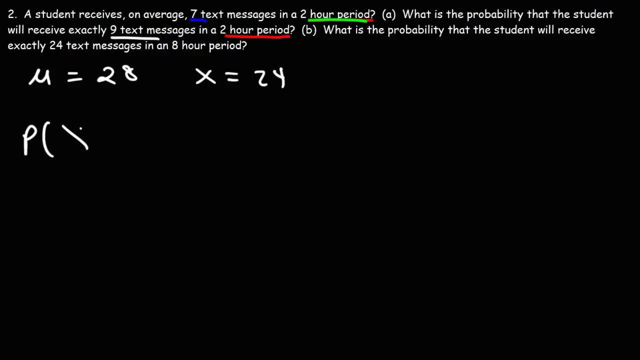 So X is 24.. So we're going to use this formula: P of X is equal to 24.. That's going to be Mu to the X. So that's 28 raised to the 24th power times, E raised to the negative Mu, which is 28, divided by X factorial. 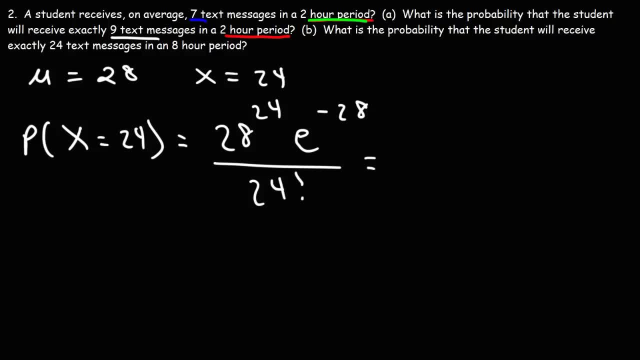 And so that's going to be 24 factorial And this is going to be. The answer I got is 0.060095.. So it's approximately 6%, Or you could say 6.01%. So that's it for question 2 of this video. 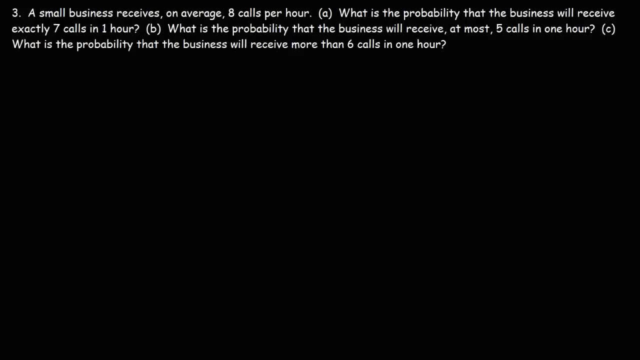 Number 3. A small business receives on average 8 calls per hour. What is the probability that the business will receive exactly 7 calls in 1 hour? So we know how to do these types of problems. So we can clearly see that the mean is 8 and X is 7.. 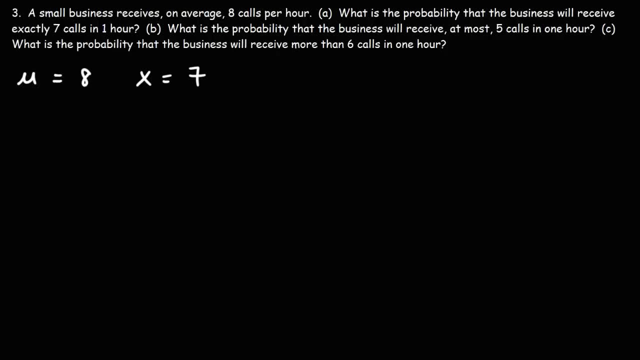 Since we want to calculate the probability when X is 7.. So it's going to be P of X is equal to 7.. And that's going to be Mu to the X. Mu is 8.. X is 7 times E raised to the negative Mu over X factorial. 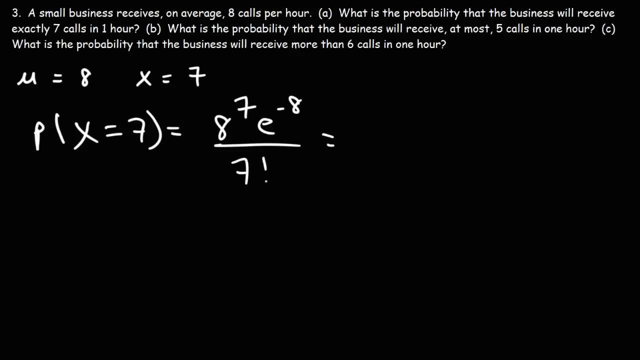 So if we plug this in, This is going to be 0.1395865.. Or we could say approximately 13.96%. So that's the answer for part A. Now let's move on to part B. What is the probability? 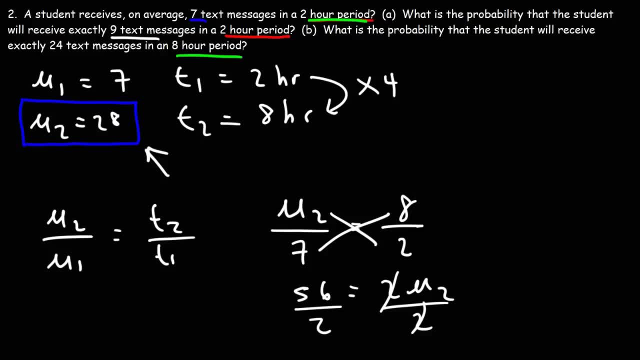 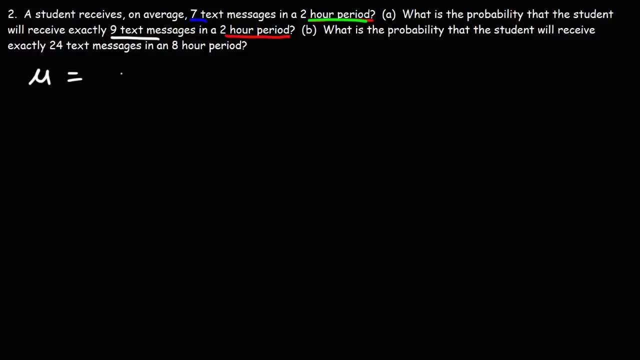 by two, which is 28.. Now let's rewrite what we know. So, mu, we could see that it's 28. And x has to be 24.. We want to calculate the probability that the student will receive exactly 24 times. 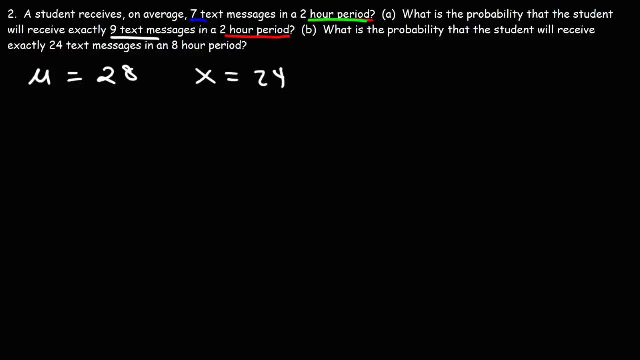 text messages in this eight hour period. So x is 24.. So we're going to use this formula: P of x is equal to 24.. That's going to be mu to the x, So that's 28 raised to the 24th power times, e raised. 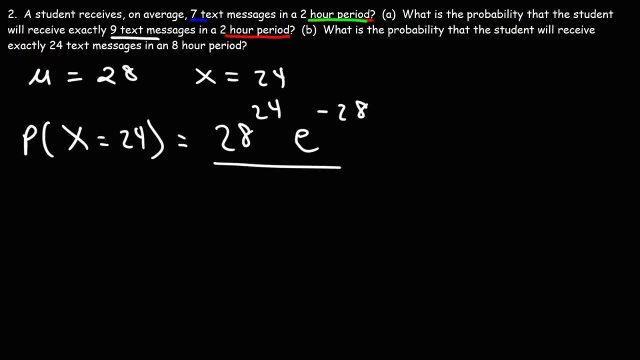 to the negative mu, which is 28 divided by x factorial, And so that's going to be 24 factorial And this is going to be the answer I got is 0.060095.. So it's approximately 6%, or you could say 6.01%. 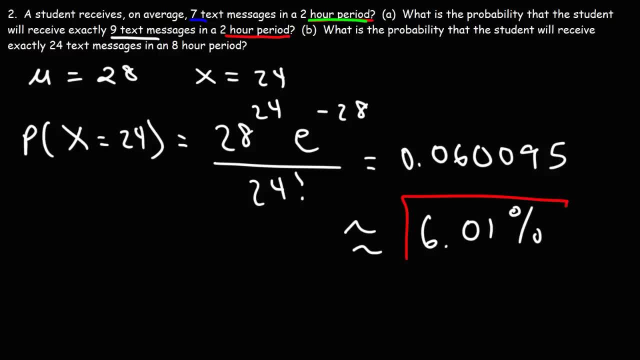 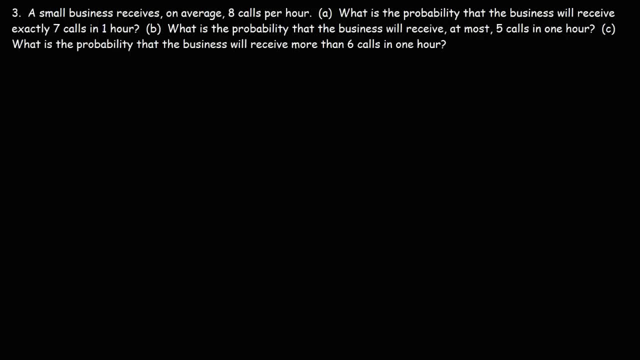 So that's it for question two of this video, Number three. a small business receives on average eight calls per hour. What is the probability that the business will receive eight calls per hour? The probability that the business will receive exactly seven calls in one hour. So we know how. 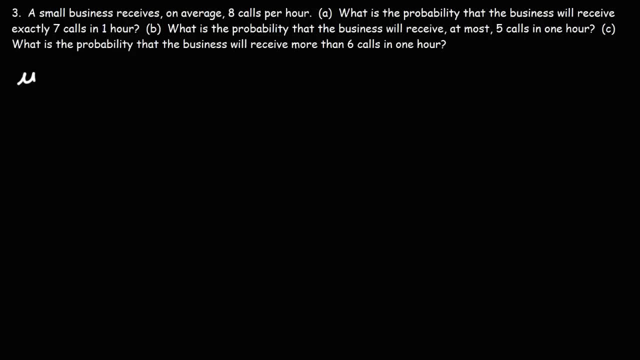 to do these types of problems. So we can clearly see that the mean is eight and x is seven. since we want to calculate the probability when x is seven, So it's going to be P of x is equal to seven And that's going to be mu to the x. mu is eight, x is seven times e raised to the negative. 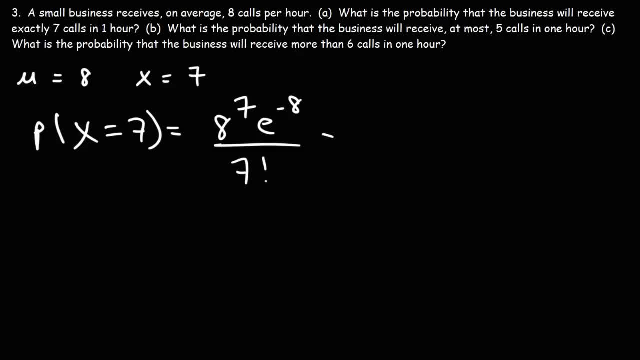 mu over x factorial. So if we plug this in, this is going to be 0.1395865.. Or we could say approximately 13.96%. So that's the answer for part eight. Now let's move on to part B. What is the probability that the business will receive at most five calls? 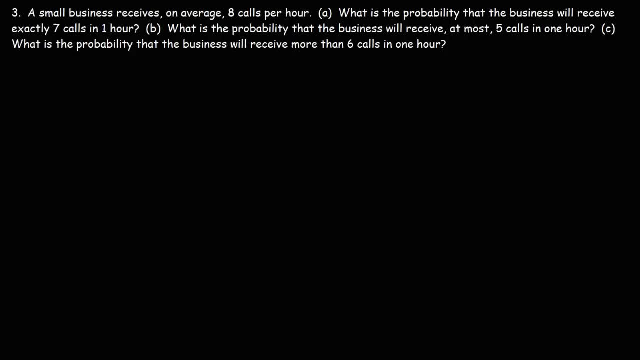 That the business will receive at most 5 calls in 1 hour. Now Mu is still 8.. That's not going to change. But what is X? X could be any number, any whole number, up to 5.. 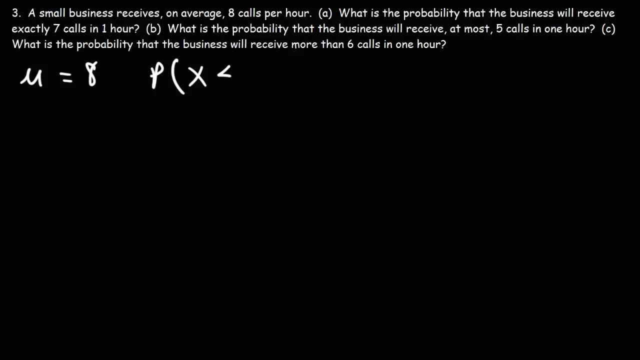 So we want to find the probability that X is less than or equal to 5.. So I'm just going to rewrite it here. So this is equal to the probability that X is equal to 0.. Now, just to conserve space, I'm not going to write X all the time. 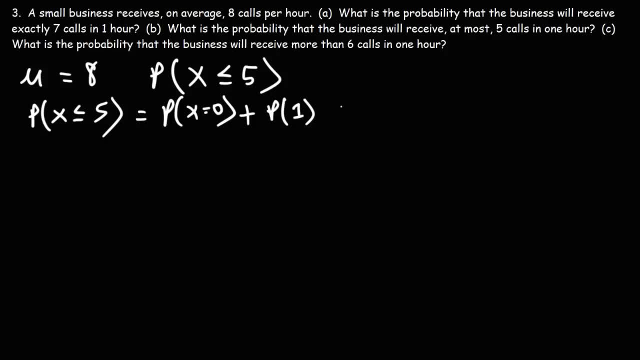 But it's going to be plus the next one where X is equal to 1, plus when X is equal to 2, all the way to when X is equal to 5.. So we have to add up the individual probability values. 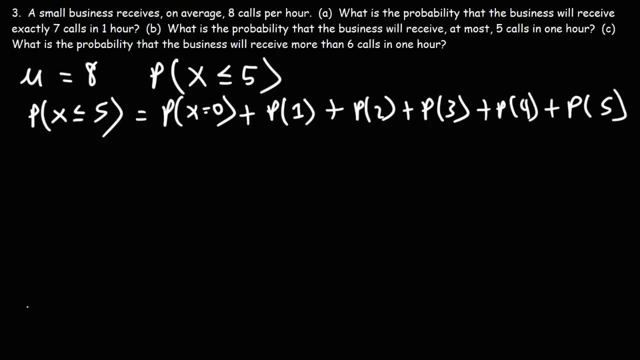 Now, fortunately, there's a quick way of doing this. I'm going to rewrite the formula to show you. So it's Mu to the X, E to the negative, Mu divided by X factorial. Now X is the variable U and E doesn't change. 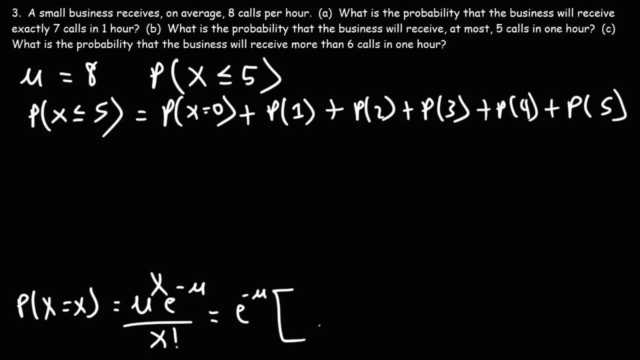 So what I'm going to do is I'm going to factor out E raised to the negative Mu and then write Mu to the X over X factorial, because that's the part of the equation that's going to change with the change in X values. 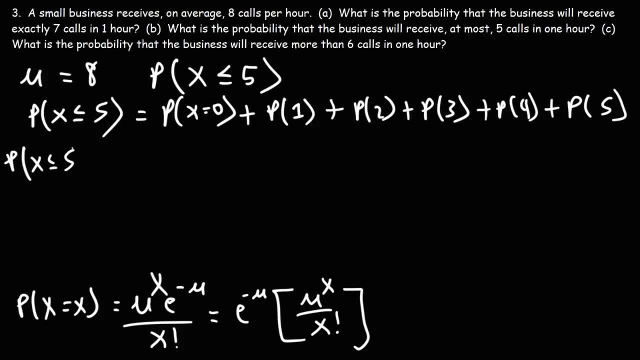 So we could say that P, when X is less than or equal to 5, is going to be E to the negative Mu, which is E to the negative 8.. And then times we're going to plug in these values when X is 0. 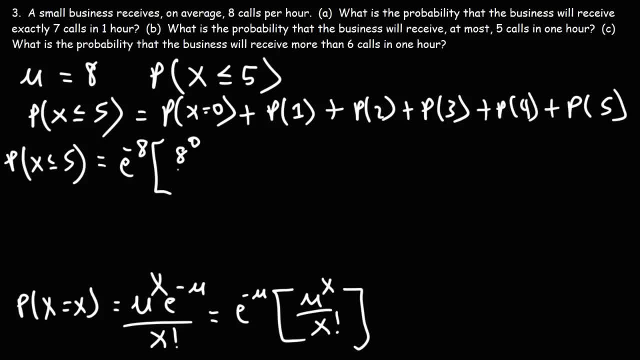 So Mu is always 8, raised to 0 power over 0 factorial Plus. now when X is 1,, Mu is not going to change, It's still 8, but X is that Mu value. And then when X is 2,. 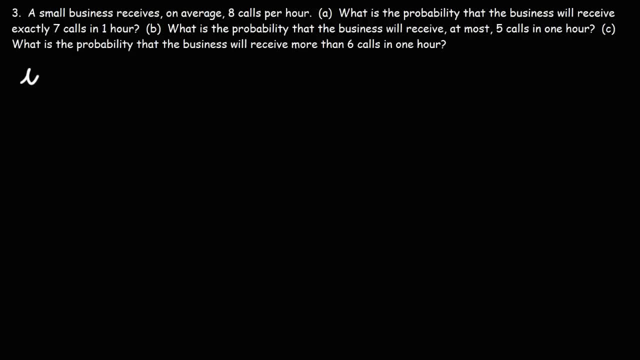 in one hour. Now, mu is still eight. that's not going to change. But what is x? x could be any number, any whole number, up to five. So we want to find the probability that x is less than or equal to five. So I'm just going to rewrite it here. 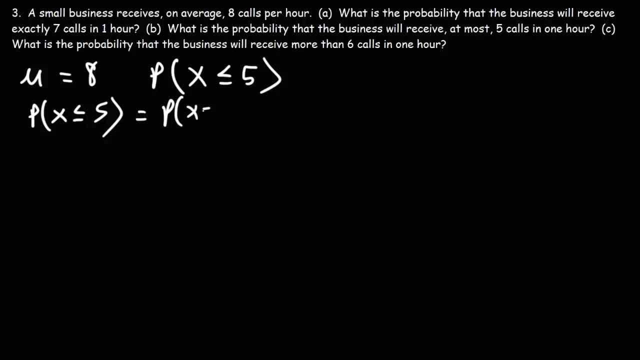 So this is equal to the probability that x is equal to zero. Now, just to conserve space, I'm not going to write x all the time, But it's going to be plus the next one where x is equal to one, plus when x is equal to two, all the way to when x is equal to five. 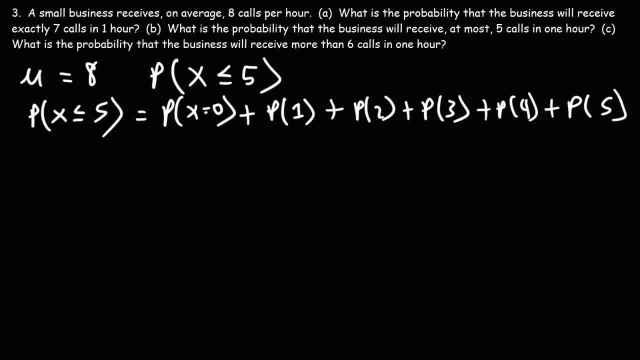 So we have to add up the individual probability values. Now, fortunately, there's a quick way of doing this. I'm going to rewrite the formula to show you. So it's mu to the x, e to the negative mu divided by x factorial. Now x is the variable U and e doesn't change. So what I'm going to do is: 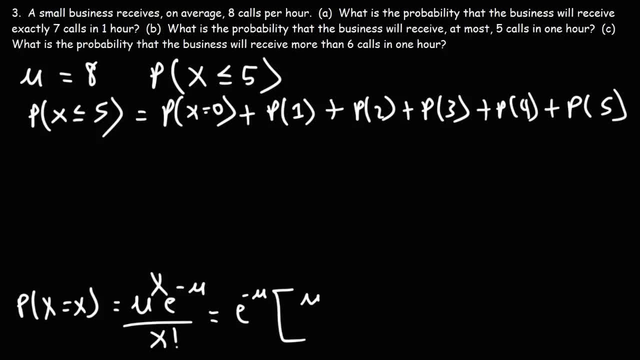 I'm going to factor out e raised to the negative mu and then write mu to the x over x factorial, because that's the part of the equation that's going to change with the change in x values. So we could say that p, when x is less than or equal to five, is going to be e to the negative. 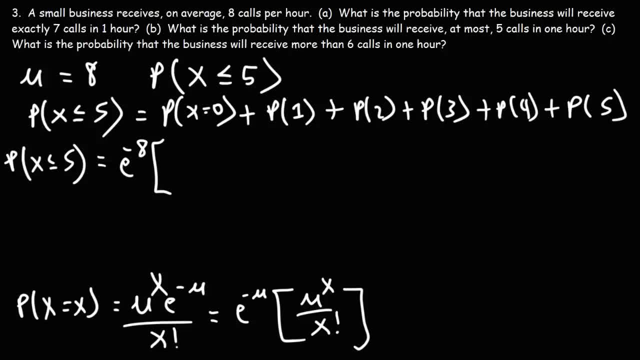 mu, which is e to the negative eight, And then times. we're going to plug in these values when x is zero, So mu is always eight raised to zero, power over zero factorial plus. now, when x is one, mu is not going to change, It's still eight. 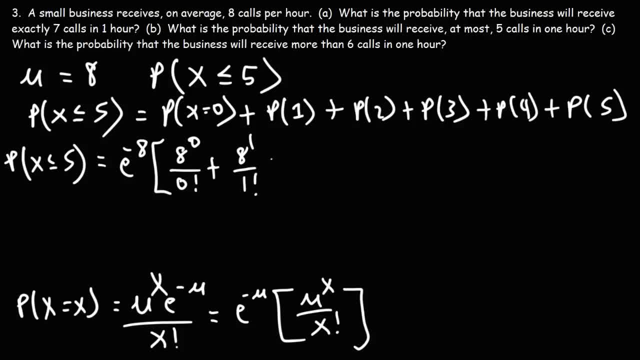 but x is that new value, And then when x is two, and so forth, And then you could just follow the pattern. So this makes it a little easier to calculate the cumulative probability values. So go ahead and type this in your calculator. 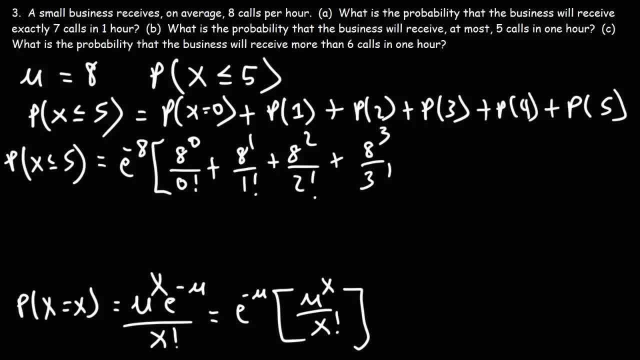 and so forth, And then you could just follow the pattern. So this makes it a little easier to calculate the cumulative probability values. So go ahead and type this in your calculator: E to the 0 is 1.. So I got 0.191236.. 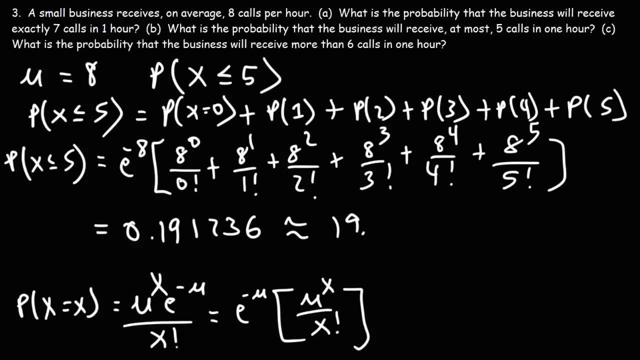 So that's a 19.12% chance that the business is going to change. So that's a 19.12% chance that the business is going to change. So that's a 19.12% chance that the business is going to receive at most five calls in one hour. 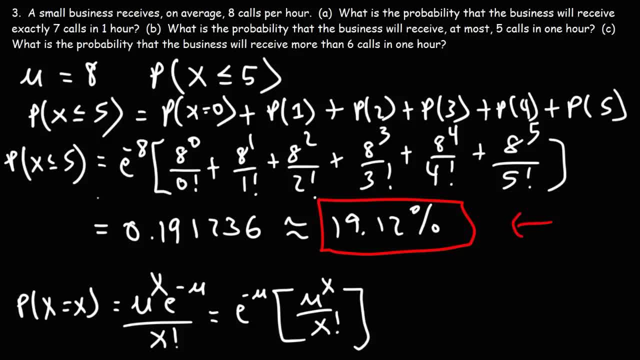 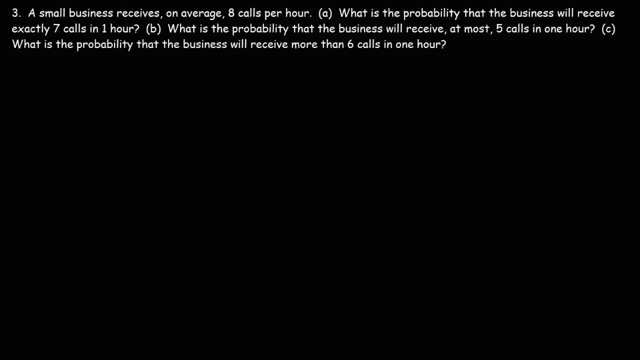 So that's it for Part B. Now let's move on to Part C. What is the probability that the business will receive more than six calls in one hour? So the time interval is still one hour, which means Mu is still 8.. 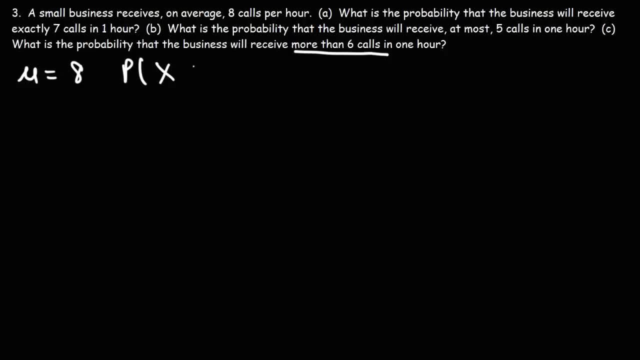 But now we want to calculate the probability that X is greater than 6, but not equal to 6.. So X could be 7,, 8,, 9,, 10, and so forth. Now this can go to infinity. 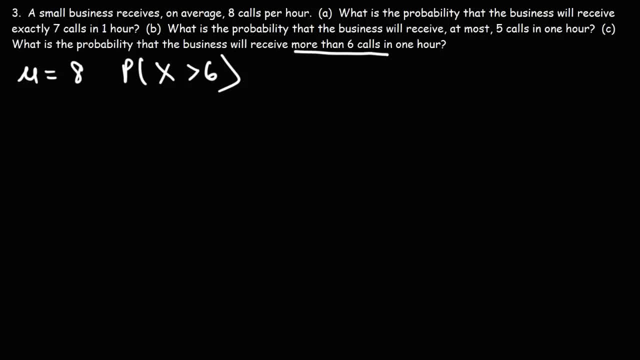 So it doesn't end. How can we find the answer in this case? Well, let's draw a picture. The Poisson distribution has a graph that is decreasing over time. The probability is on the X, I mean it's on the Y- axis. 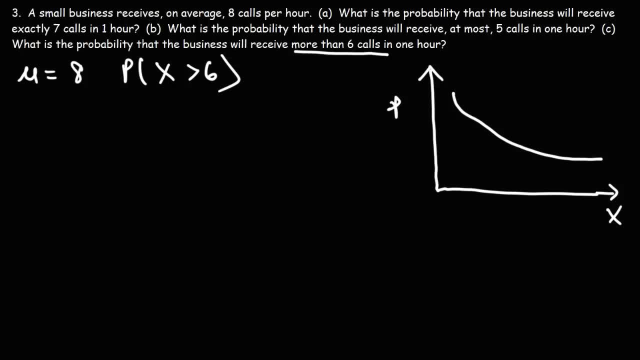 the random variable X is on the X axis or the horizontal axis. Now let's say X is 6 at this point. So we're going to split the graph into two parts. Let me use a different color. Now let's say that the probability of the student receiving 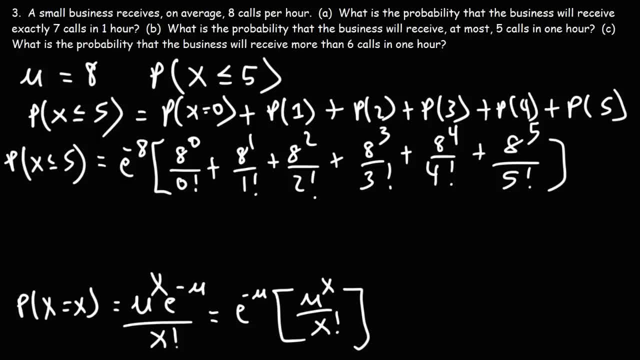 Eight to the zero is one. So I got point one. nine, one, two, three, six. So that's a a 19.12% chance that the business is going to receive at most five calls in one hour. So that's it for part B. Now let's move on to part C. 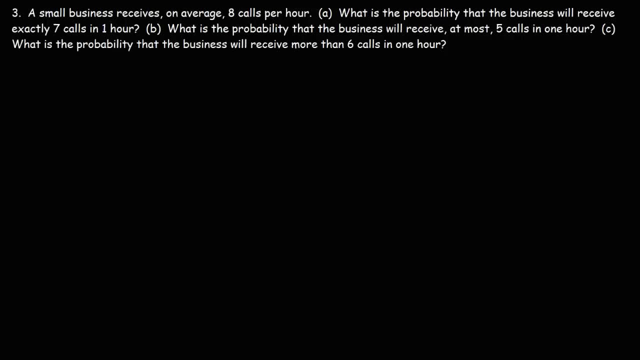 What is the probability that the business will receive more than six calls in one hour? So the time interval is still one hour, which means mu is still eight. But now we want to calculate the probability that x is greater than six, but not equal to six. 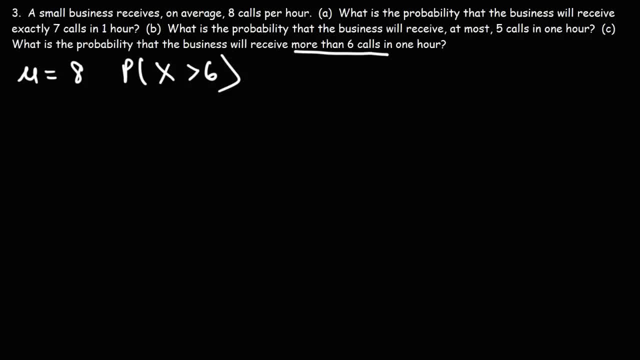 So x could be seven, eight, nine, ten and so forth. Now this can go to infinity, So it doesn't end. How can we find the answer in this case? Well, let's draw a picture. So the Poisson distribution has a graph that is decreasing over time. 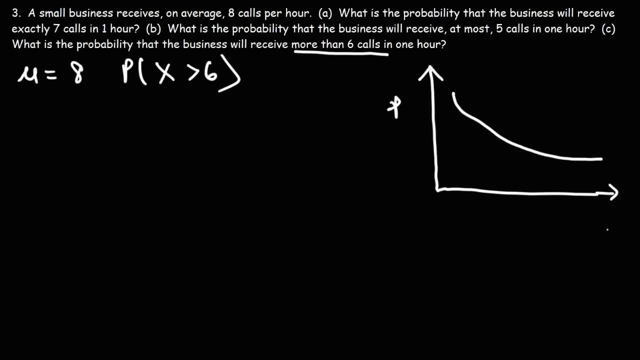 The probability is on the y-axis, The random variable x is on the x-axis or the horizontal axis. Now let's say x is six at this point. So we're going to split the graph into two parts. Let me use a different color. 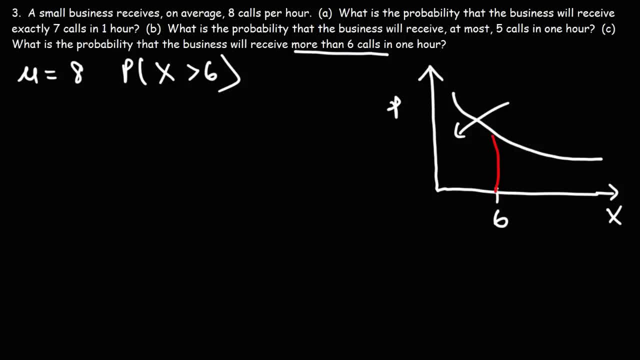 Now let's say that the probability is six at this point. So we're going to split the graph into two parts. So let's say the probability of the student receiving, let's say the probability that the business receiving six or less calls is 30%, just to give a number for the sake of illustration. 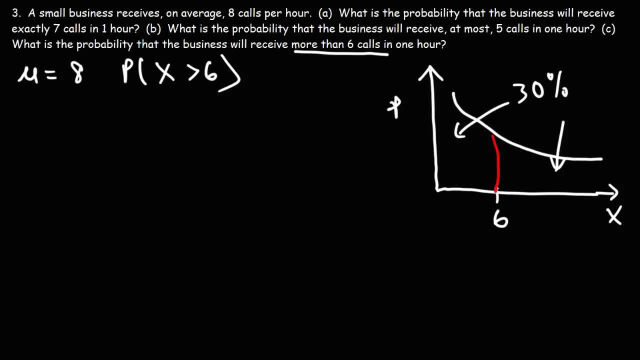 What is the probability that x will be greater than six? The total area under the curve, which represents the total probability, is one or 100%. So if the probability that x is equal to or less than six, if it's 30%, then the probability that x is greater than six will be 70%, because these two have to add. 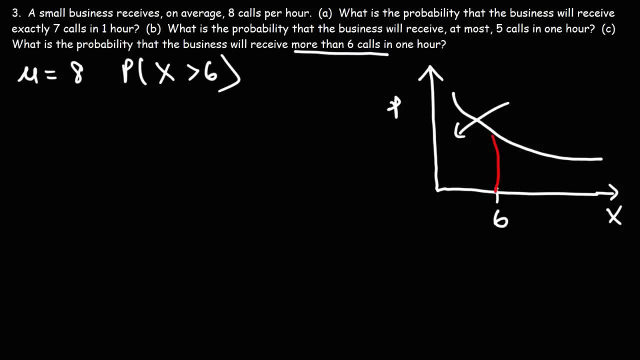 let's say the probability that the business receiving six or less calls is 30%. Just to give a number for the sake of illustration. What is the probability that X will be greater than 6? The total area under the curve which represents the total probability, is one or a hundred percent. 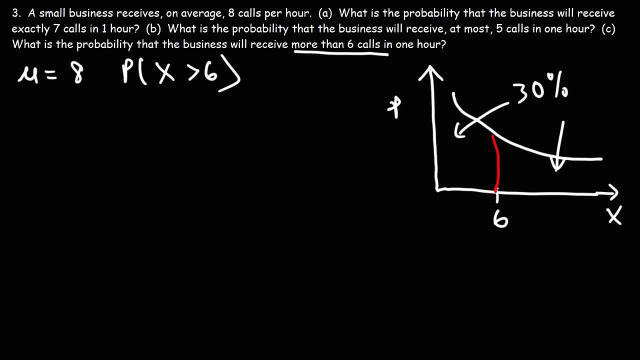 So if the probability that X is equal to or less than six, if it's 30%, and then the probability that X is greater than six will be 70%, because these two have to add up to a hundred. So on the left side, 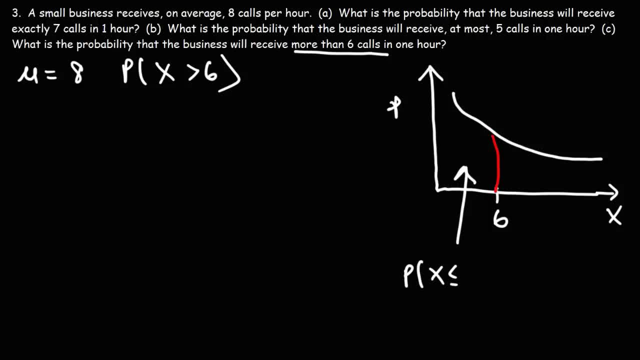 this represents the probability that X is less than or equal to six. on the right side, This represents the probability that X is greater than six. Now, if we add these two values, this is going to equal one. So if we take this term and move it to this side, 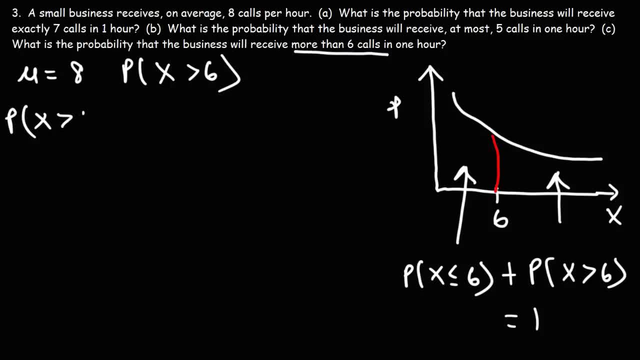 we could say that the probability that X is greater than six is one minus the probability that X is less than or equal to six. So this is going to equal one minus the probability that X is zero, plus the probability when X is one all the way up to six. 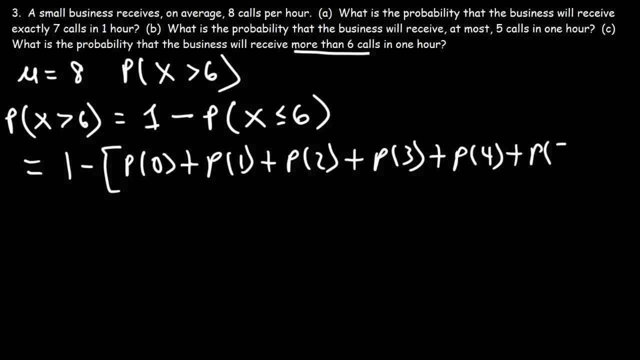 Okay, and I'm running out of space. So this is going to be one minus. We're going to use the same procedure that we did in part B, So it's E to the negative eight and then times mu zero, I mean. 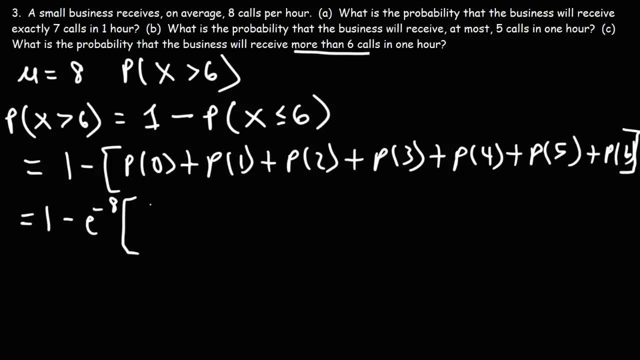 mu to the X over X factorial. So mu is still eight, X is zero. and then plus eight to the first power over one factorial, plus eight, So the second power over two factorial. and we're going to repeat this until we get to six. So go ahead and type this in: 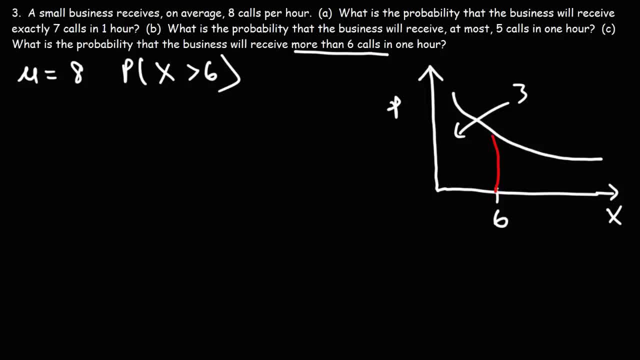 up to 100.. So on the left side, this represents the probability that x is less than or equal to six. On the right side, this represents the probability that x is greater than six. Now, if we add these two values, this is going to equal one. 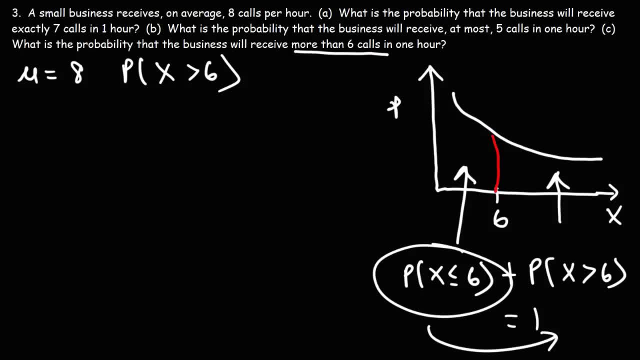 So if we take the probability that x is greater than six, this is going to equal one. So if we take this term and move it to this side, we could say that the probability that x is greater than six is one, minus the probability that x is less than or equal to six. 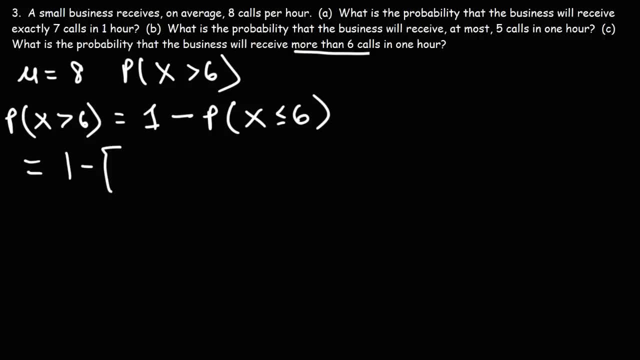 So this is going to equal one, minus the probability that x is zero, plus the probability when x is one, All the way up to six, And I'm running out of space. So this is going to be one minus. we're going to use the same procedure. 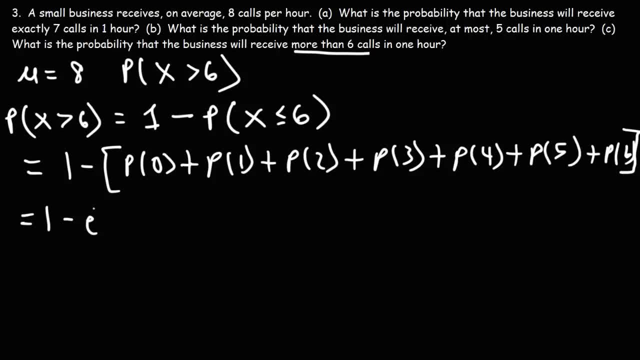 that we did in part B. So it's e to the negative eight and then times mu, zero. I mean mu to the x over x factorial, So mu is zero and mu to the x over x factorial, still 8, x is 0, and then plus 8 to the first power over 1 factorial, plus 8 to the second. 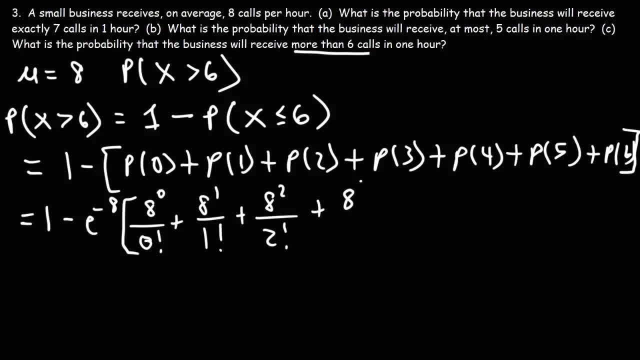 power over 2 factorial, and we're going to repeat this until we get to 6.. So go ahead and type this in. Hopefully you have a scientific calculator which will make life a lot easier when dealing with problems like this. So I got 0.686626, so we could say that it's approximately a 68.7% chance that the business